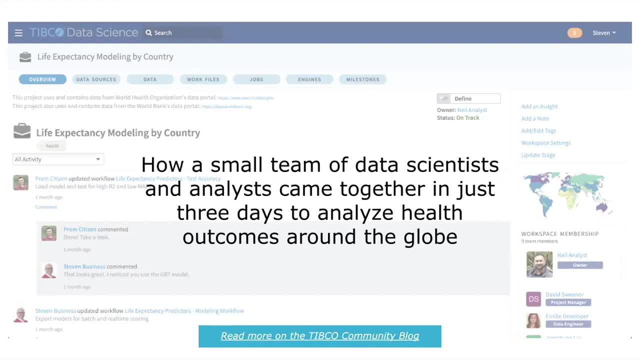 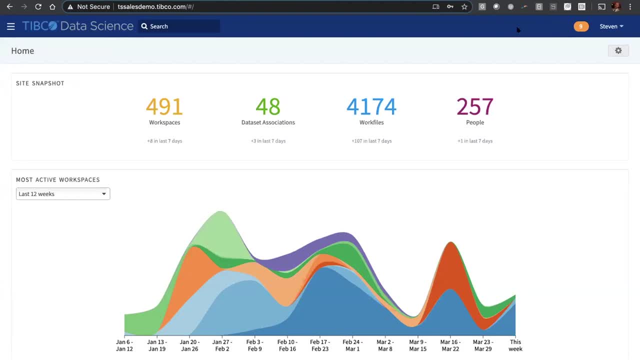 But I think it'll amply demonstrate the sort of personas that Michael was just talking about. So let me switch to the live demo Here. you see, I'm logged in- as myself, In fact- to our- Okay, So this is our TIBCO data science platform and this is not a fake system. 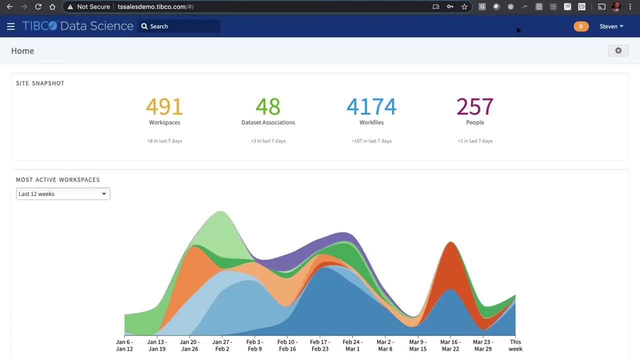 This is actually where we run most of our analytics projects, including the one that I was just talking about, And you can see, just a few weeks ago there was a little spike of a few days where part of my team was focused on modeling life expectancy for countries around the world. 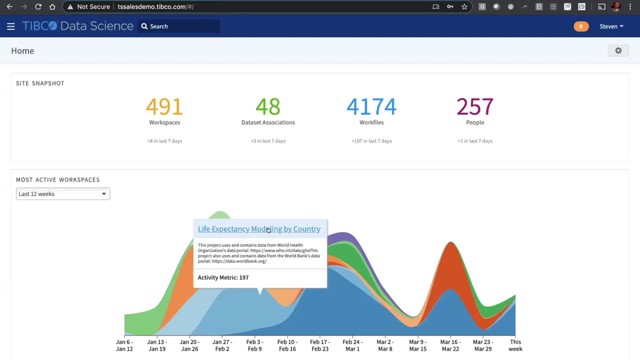 And so you can see the spike of activity Really over the course of three or four days. the team came together because we sort of learned about the challenge a little bit later. we didn't have much time to work on it And actually we sort of turned that back. 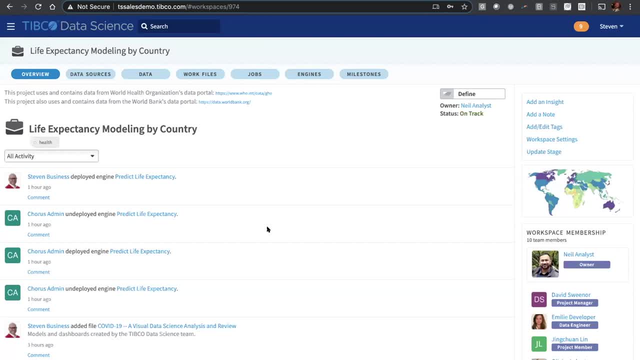 And so I think it's really important to think about how can we bring that to our advantage, How can we rapidly bring a team together to produce some meaningful analytics as quickly as possible? So here in this workspace, everything in the TIBCO data science world is divided into project. 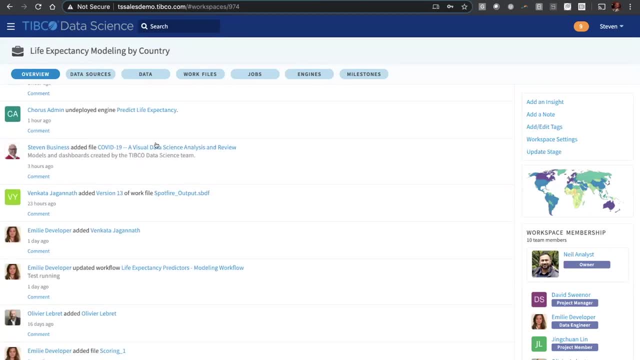 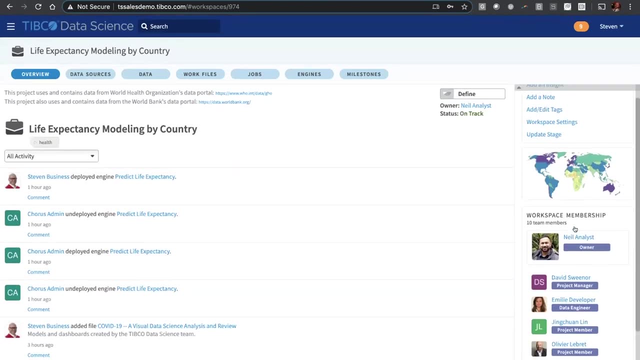 workspaces And you can see the recent activity here, including that blog that I was just mentioning on the current outbreak, which I added to this workspace. But, again, by going back to this particular analysis, this was the team that was working on it. 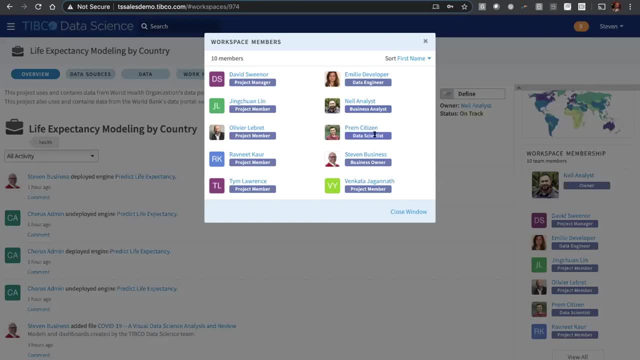 If I look at the team in general, you'll see we've got here a data engineer, business analyst engineer. I've got a data scientist myself as the owner of the project listed out, as well as some other people who are just sort of auditing. 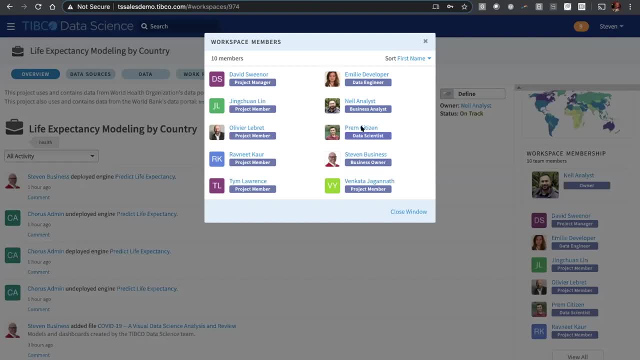 And that's really what I want to call out as I go through the demo- is how these different personas interacted with each other. We even actually changed our names just to call out the roles that we were playing. So you'll see, I start out in the persona of Neil, who is our business analyst, who is 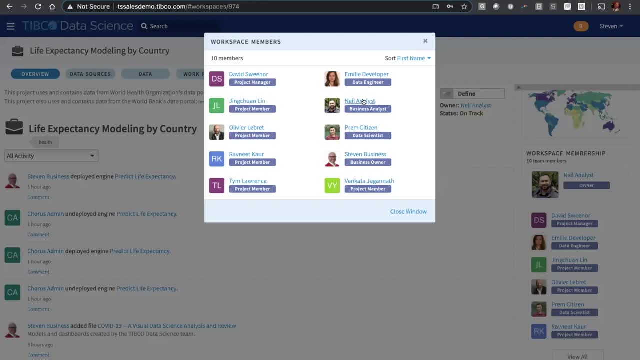 working with Spotfire to do some initial data wrangling, get the data prepped and come up with some initial insights, before he then passed off And then I handed off to me to sort of set up the data science side of the project and 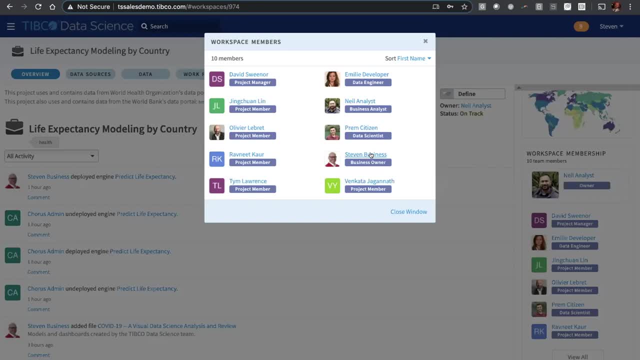 do some very basic analysis as sort of a business owner, And then I handed off to Prem, who is our data scientist, perhaps what one might arguably call a citizen data scientist or a data analyst, who then did some preliminary modeling with some assistance from Emily, a machine learning engineer or data engineer, who was doing some 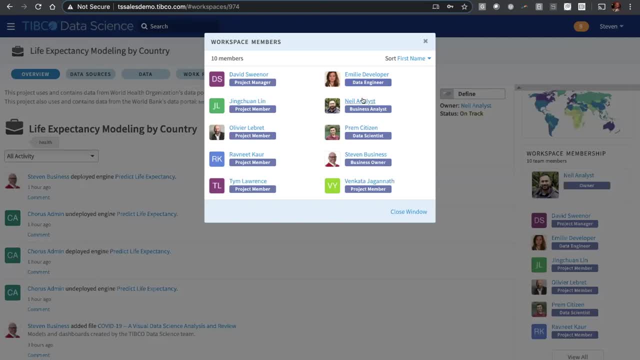 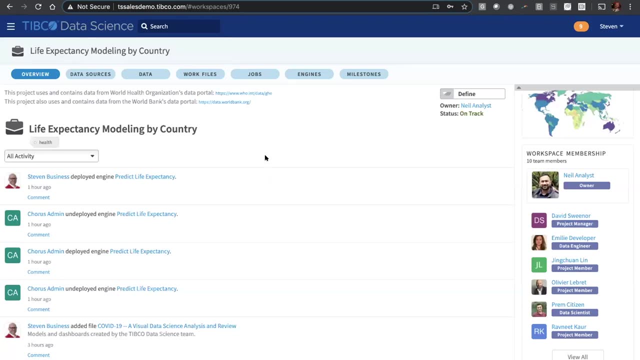 work in Python, before we then yielded the results back to Neil for review in Spotfire. So this is the little team that was working together and, as I say, just in a few days we produced something that you're now about to see. 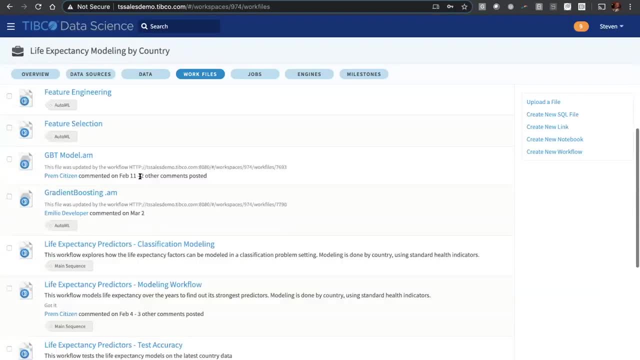 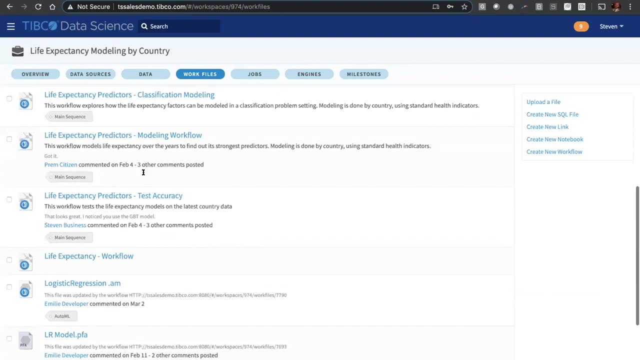 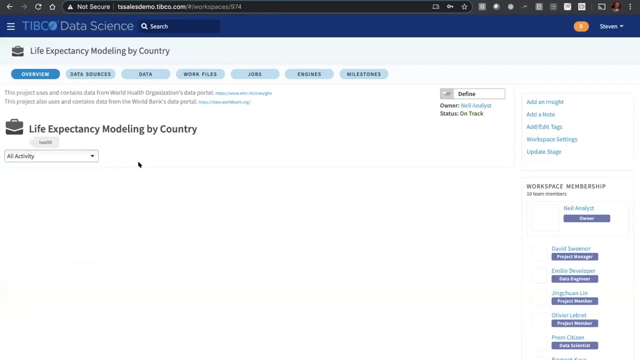 All of our work is collected here together in the work files area. So you see here visual workflows, Python SQL notebooks, predictive models that we've exported, links to Google Sheets and so on. Pretty much everything is collected here And then sort of audited over time through this sort of interactive activity stream. 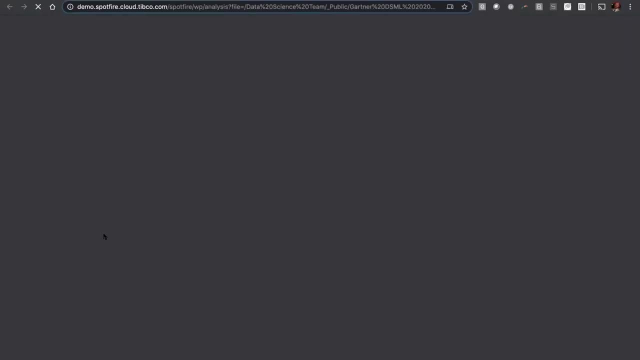 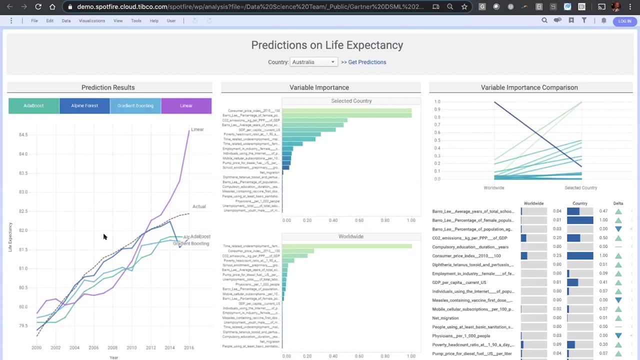 Let me focus, to start with, on the dashboard that Neil created as the business analyst. This is in Spotfire, running on the web. In fact, everything you're seeing here is running in cloud. It can also run on premise, of course, but here we're running everything on Amazon and 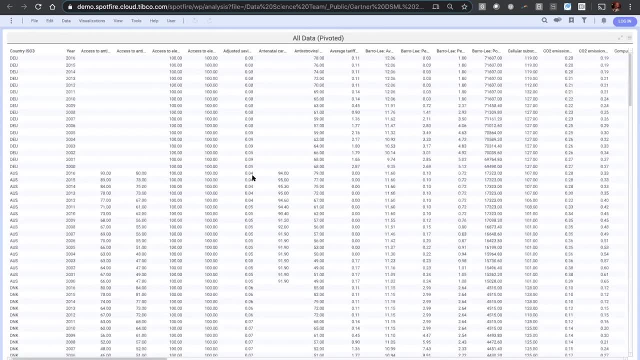 using Amazon data sources. And so here's what Neil started with. he did some basic pivoting and unioning of data sets to get a comprehensive view. So we started with a really comprehensive data set. We decided because the data set was relatively small, we wanted to bring in data from really 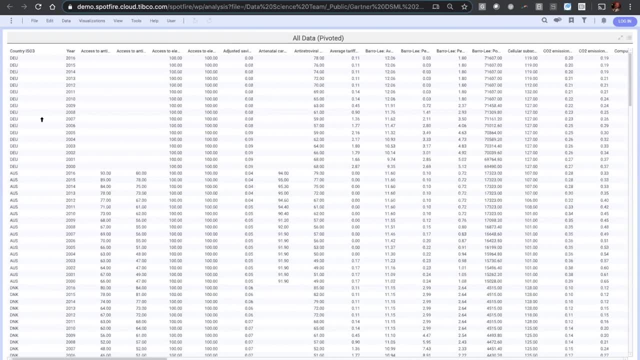 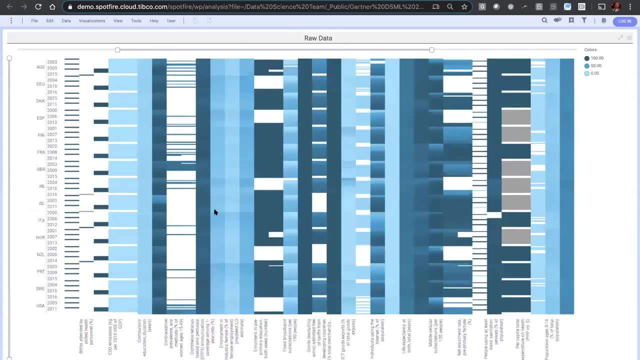 around the globe and not just focus on the initial area, which was Australia and New Zealand, And so we'd have just more data points. So there's the data. We found that there were a lot of missing values. Spotfire automatically actually pointed that out to us and made some suggestions about. 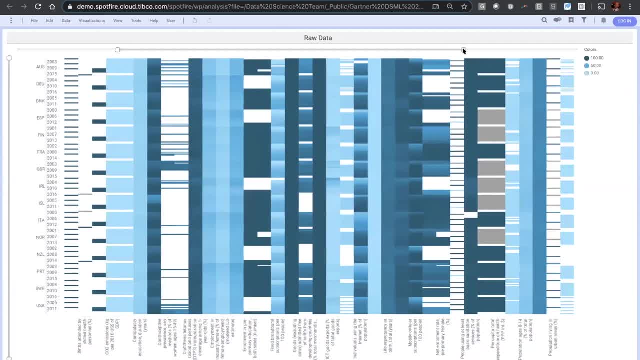 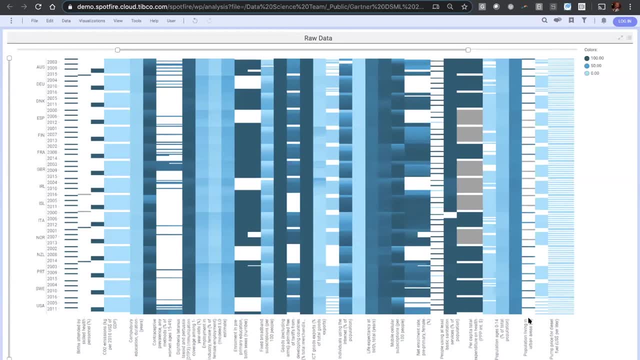 charts that we could look at in order to dig further. If you see, here, for example, there's a nice little chart showing these missing values that Neil endeavored to fill in, You'll see. for this, For example, there's a potentially quite useful variable here about population living in urban. 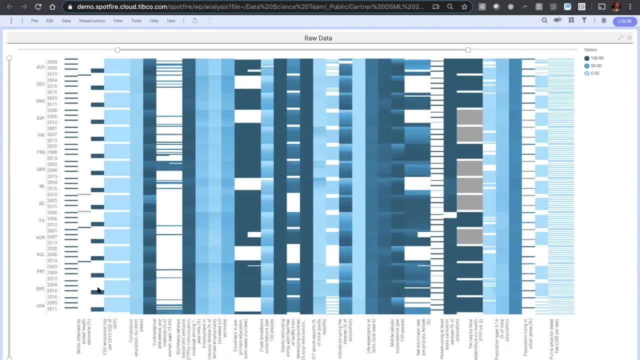 areas, but really very little data across the different countries and across the years. It went from 2016,. contraceptive usage, economic factors, trading factors and so on, as well as the actual variable that we're interested in: life expectancy at birth. 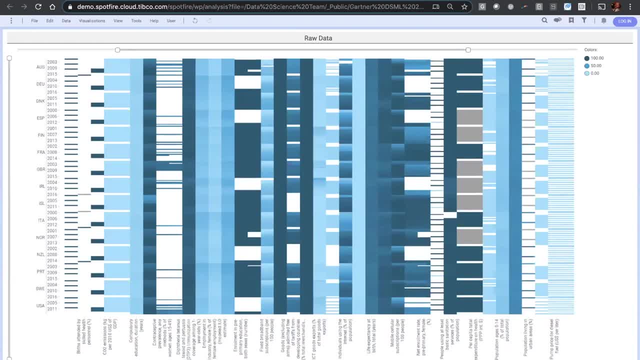 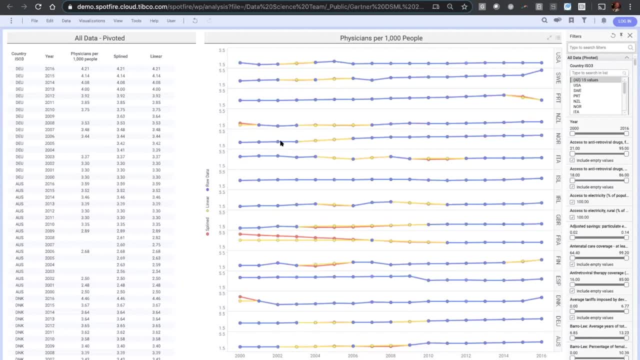 And fortunately, there you can see, there were no missing values. We looked at a variety of different methods of filling in those values. Here's the data. Here in Spotfire, we can actually use some R code embedded within our dashboards to fill. 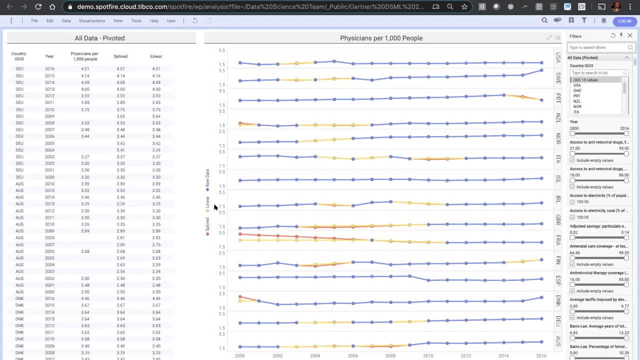 in missing values using basic interpretation like linear interpolations, more advanced methods using splines. We decided to stick with linear. It actually seemed to give pretty good results. It was quite simple, And so, having done that, Neil was then able to fill in the missing values here. 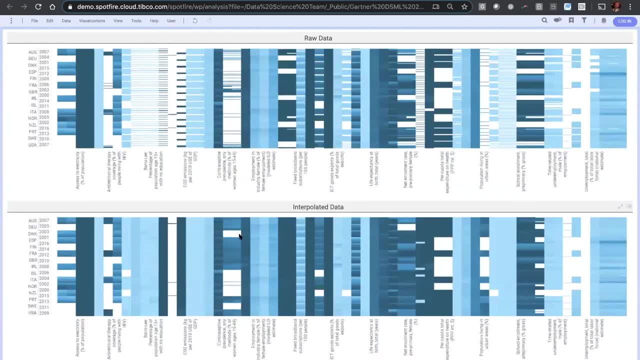 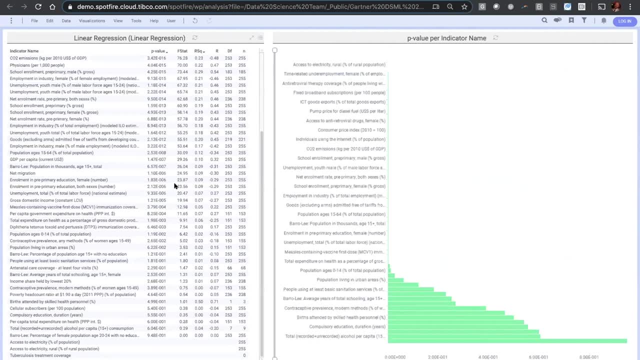 You see the results. There's still some where you just don't even have enough data to interpolate, but it's much more comprehensive and rich data set now. Neil then sort of started playing around with this. He looked at perhaps some initial measures of variable importance using a basic regression. 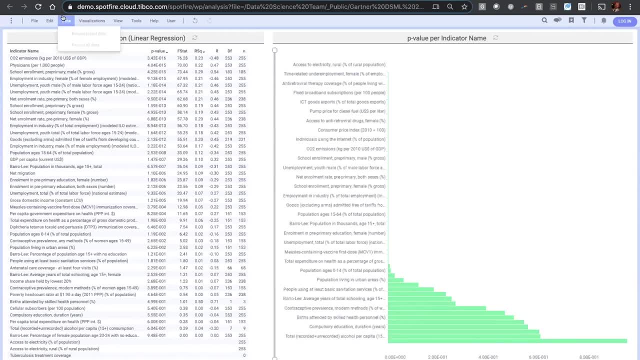 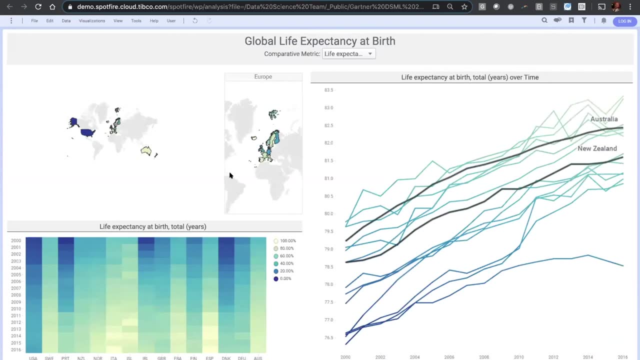 that's built into the data relationships tab within Spotfire. He also built a basic dashboard here just looking at different countries and looking at- He's also looking at the values of life expectancy just to get a broad sense of what was happening from country to country. 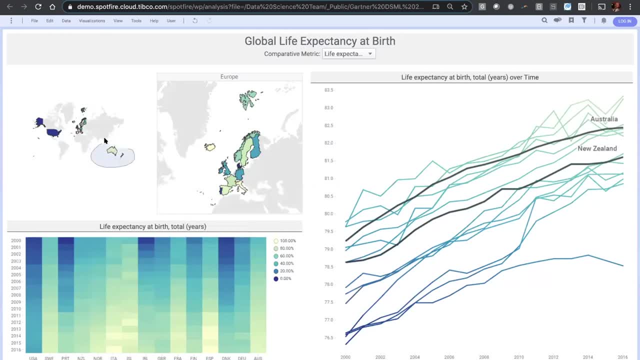 Again focusing here on Australia and New Zealand, so I can sort of isolate that in the map here, just to call that out. I can look across different countries. See here the Nordic countries, perhaps not surprisingly having particularly high percentiles in terms of longevity. 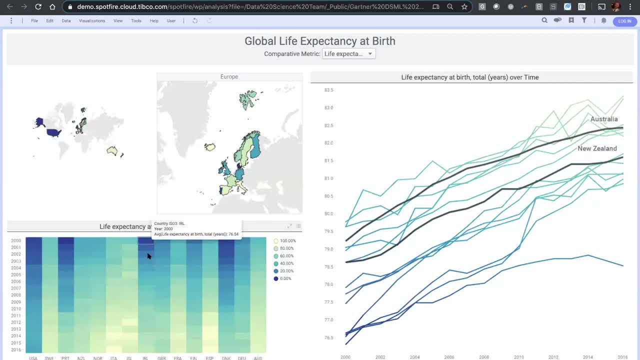 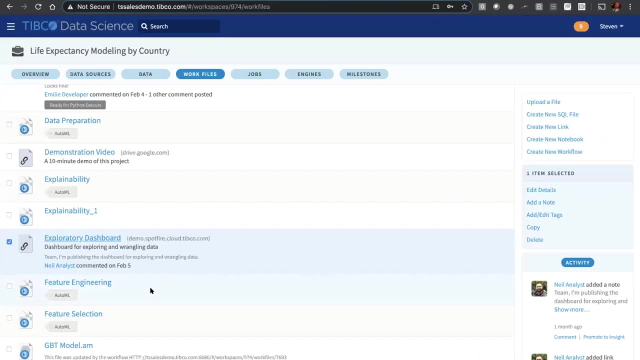 Significant improvement over the 16 years: 17 years for Ireland, but still a significant improvement. And then you can see in the map here the numbers Ireland. But at this point Neil decides to hand over to the data science team to do a more advanced. 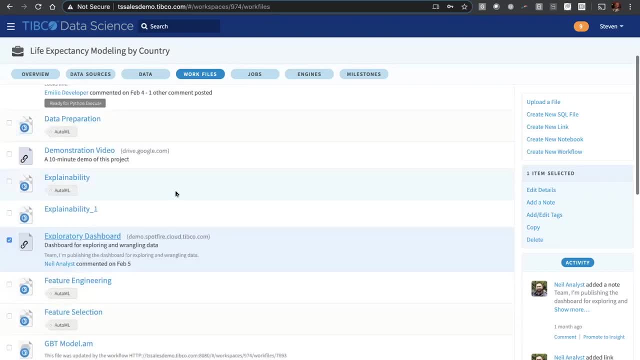 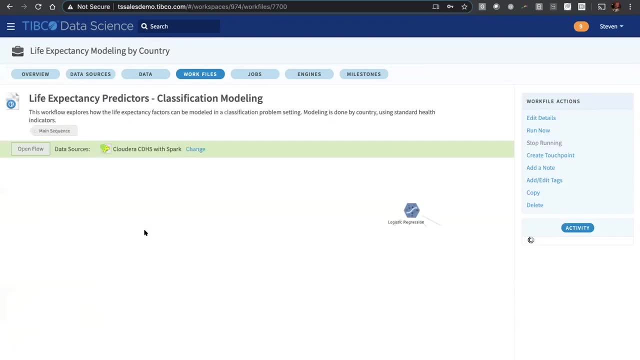 analysis. So that's where I come in to sort of set up this project. I create this workspace link back to the Spotfire dashboard from within here And I actually created a very simple. so think of me as sort of the idiot manager doesn't know what he's doing, but can do some. 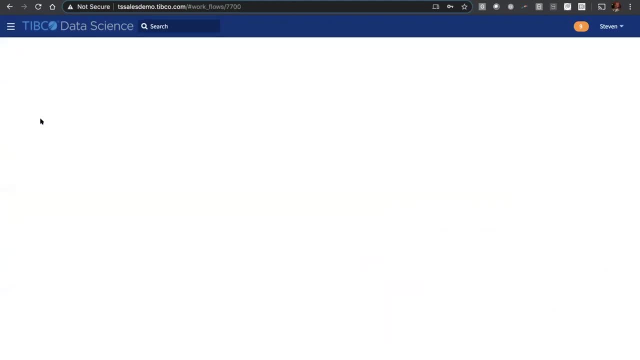 basic stuff here using this visual workflow. So I'll open this up And what I did is I did a very simple classification. We just said let's look at a histogram of life expectancy and see if there's sort of a cutoff point for countries that are doing well and not so well, And we'll just do. 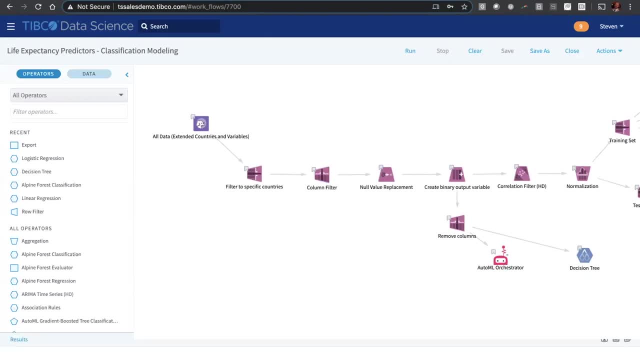 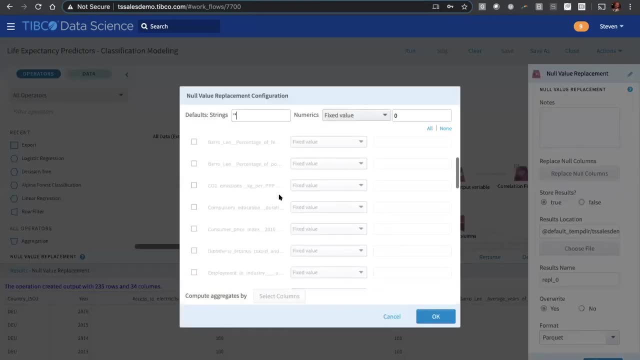 a binary classification. So that's what we do in some of these simple steps here, And I was able to do this no coding required here. So, for example, if I want to fill in some additional missing values, I can just check those here and pick whether to use a fixed value or an aggregate. 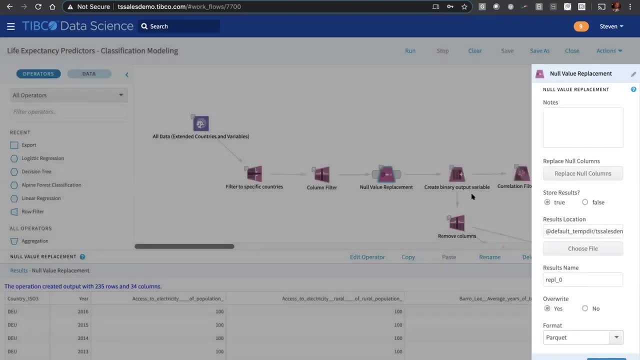 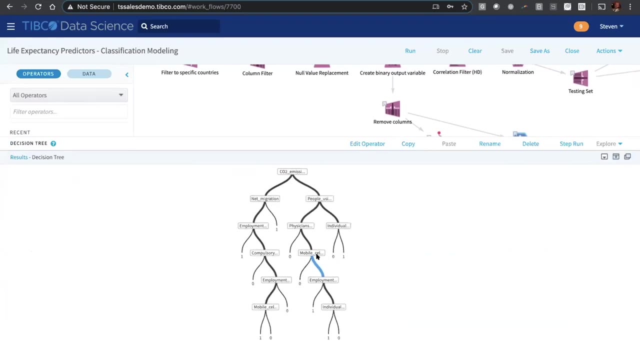 or a median, for example. Very easy for me to do that: create a binary outcome variable And then do some basic modeling. For example, here I built a simple decision tree to look at some what variables might be interesting for this particular analysis. Also, I used our 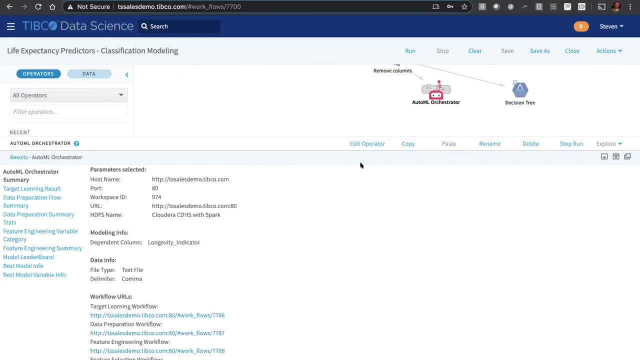 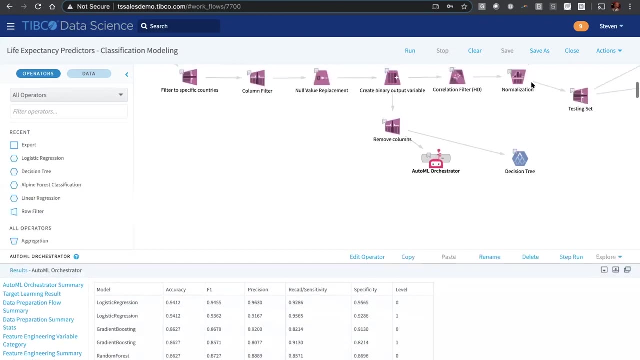 AutoML orchestrator. This is a really great feature that allows me to take something like a binary variable and build an automatic model, build a set of classification models automatically and get a leaderboard at the other end. that just shows me now which are the best models Here. 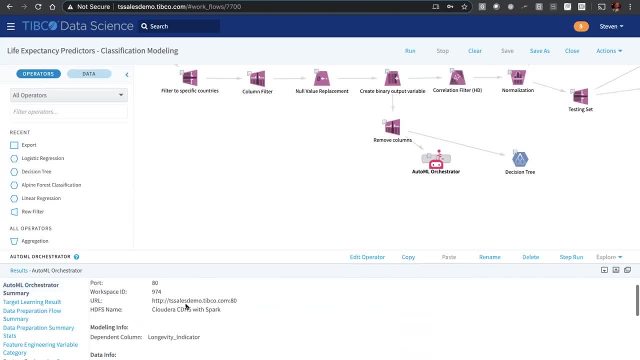 it's actually recommending a logistic model And it'll actually produce for me a comprehensive set of explicit workflows, so that it doesn't just give me a model and a recommendation and a set of statistics. It actually constructs the entire workflow from data access to data prep, to features, feature selection, modeling, even out to 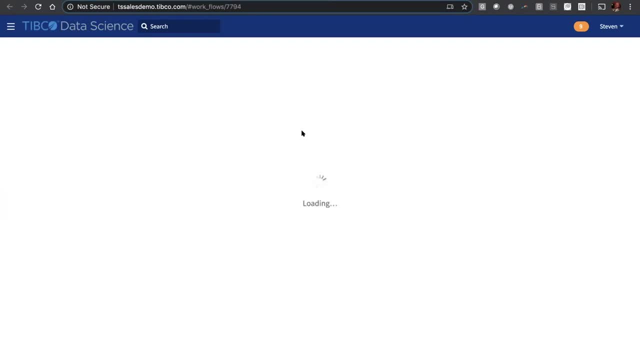 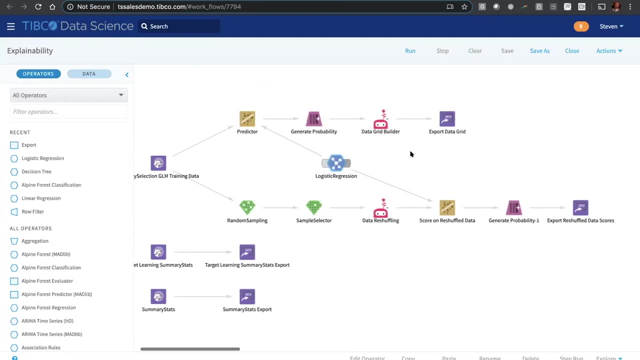 explainability. We even have an entire workflow built out that not only strings together all of the best transformations and models that the AutoML finds, but then actually builds some explainability and pushes that back to Spotfire So you can get a sense of not just which 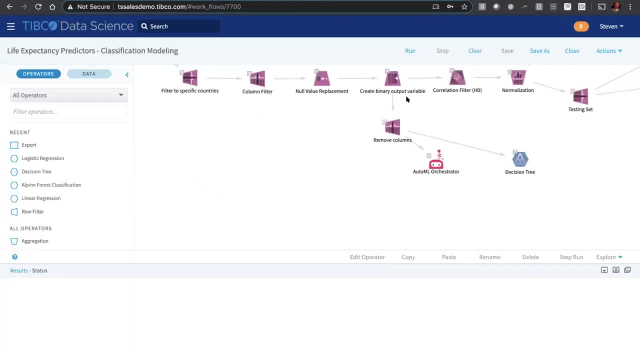 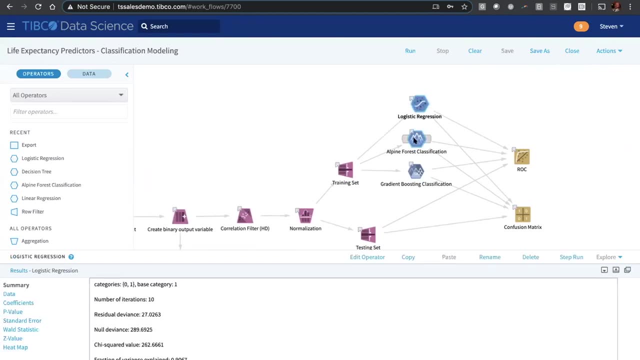 models are best, but also why they're best. That's the AutoML. Again. very easy for me to do that as sort of the business lead here. I can also build without any coding just some basic classification models here. use standard techniques like ROC curves and confusion matrices to figure out which. 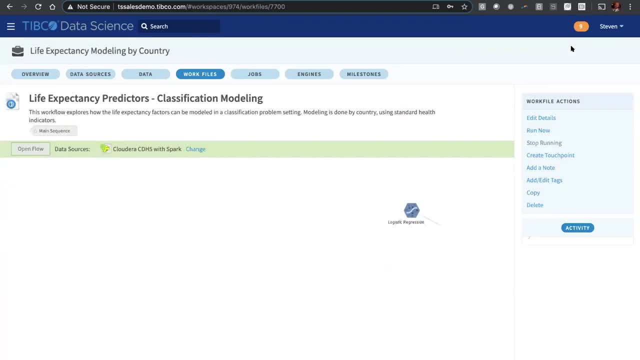 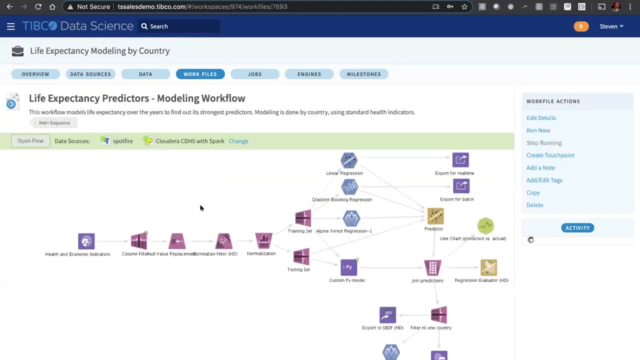 ones are doing well. But I've sort of reached the limit of my expertise here, So I'm going to hand off to a real data scientist, Prem, and this is the workflow that Prem created. This is a full modeling workflow. We're actually going to predict life expectancy here, so numerical regressions He got. 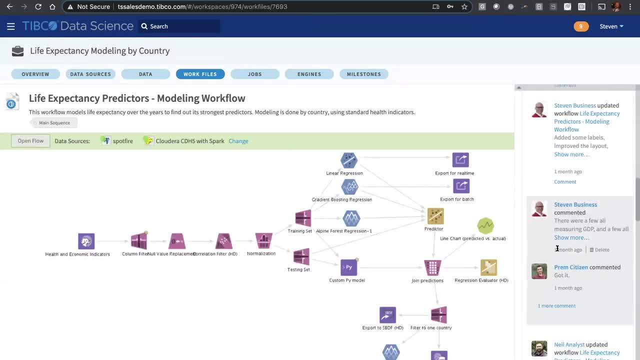 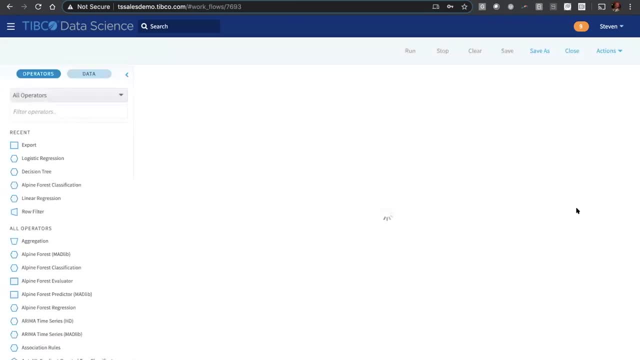 some help here from the rest of the team. As I mentioned, Emily created some Python notebooks and I sort of contributed some ideas, as well as Neil some findings from his dashboard. Let me open up and just show you briefly what Prem did in his workflow. You'll see there are 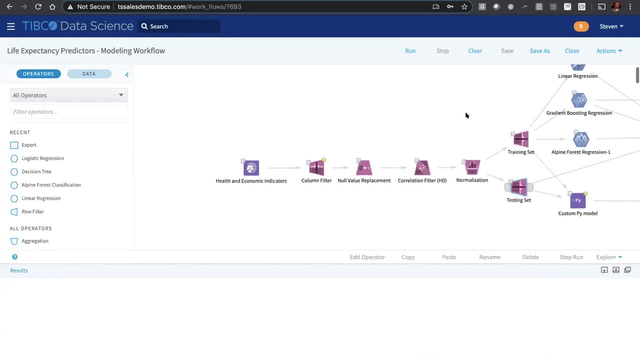 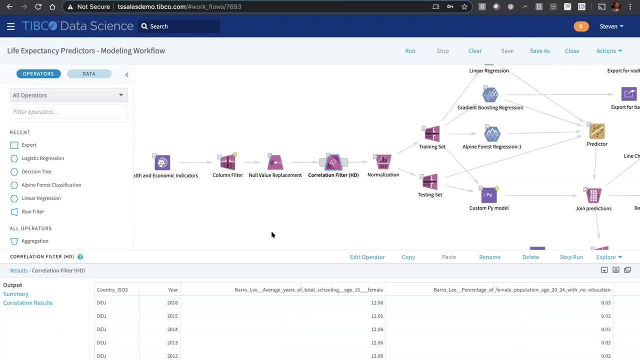 some other workers using this right now. So we did similar process of data munging up at the beginning of the workflow. We use a method called correlation filter, which we really like to use, which basically says: look, there are actually. 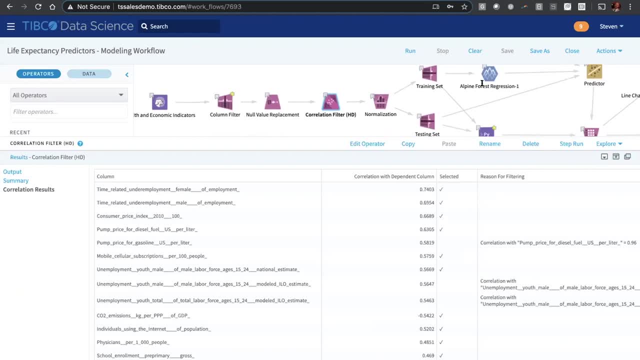 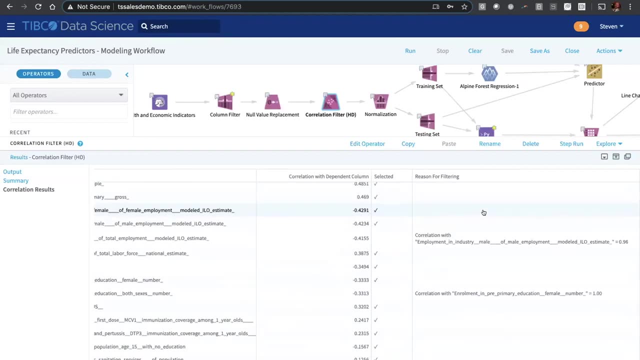 I think hundreds of socioeconomic factors that were in this data set. So we need to trim those down a little bit, And we use various techniques for doing that. One of them is just simply to look at any variables that are strongly correlated with each other. Some of these employment variables: 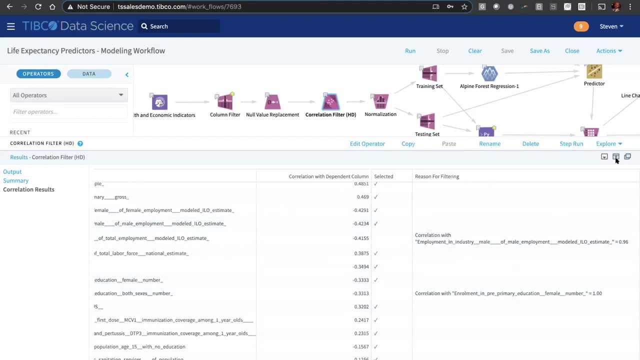 for example, sometimes have actual perfect correlations. So we just throw those out of the data set and pass that on to the rest of the workflow And then we'll get back to the final process, which is to go back to the smaller set to simplify things and make things. 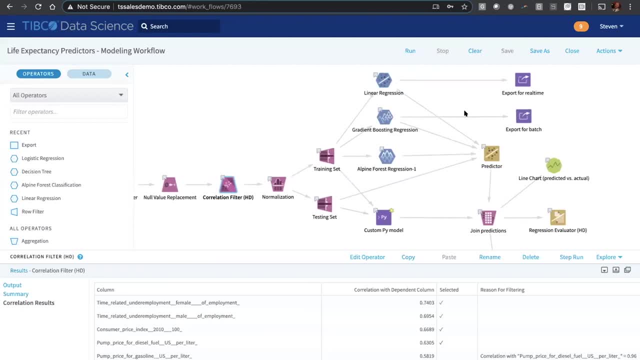 easier. So we've done that for a couple of examples, but it's not going to do any help internally. But for example, here it takes a couple of seconds or so for the business analysts to review which things were most important. Then we do standard things like 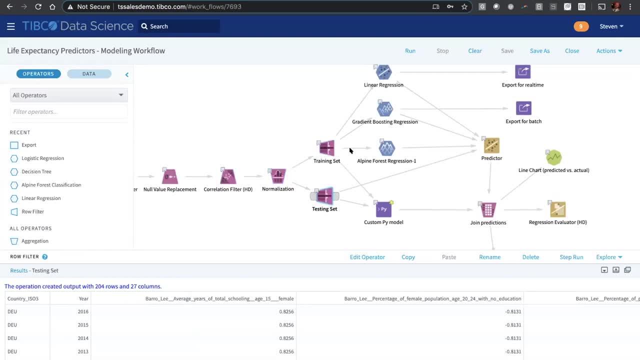 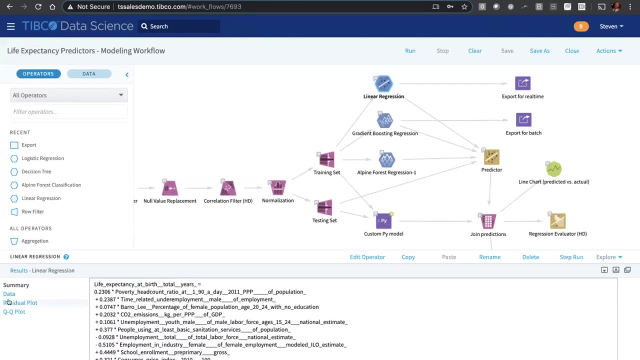 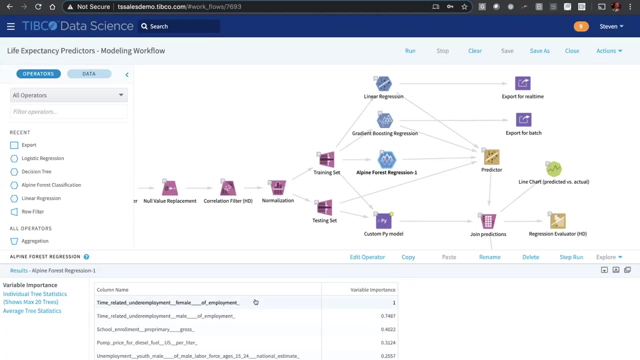 normalization split into a training and testing set based on time variable. And here we're not building classification models but actual regression models. So you can see here the linear regression with its residual QQ plots and gradient boosting, some ensemble methods- here random forest as well- yielding variable importance. 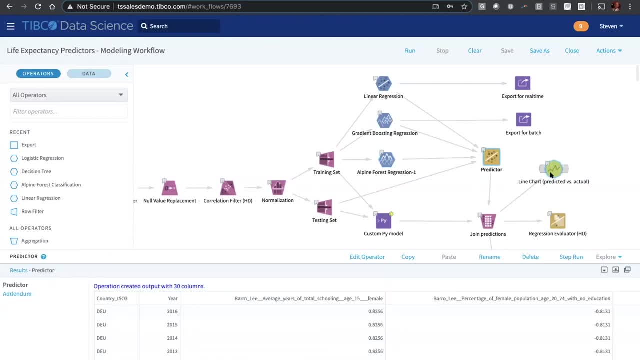 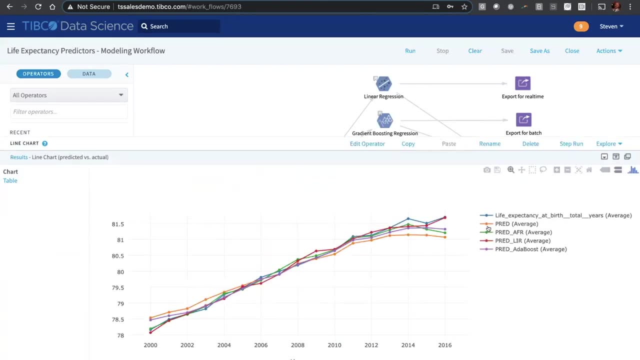 We build that model, run some predictions, build a regression evaluator to analyze some statistics about which model is best. We also look at predicted versus actual charts. I think we found in this particular case- this is analyzing all data from all countries- the linear regression. 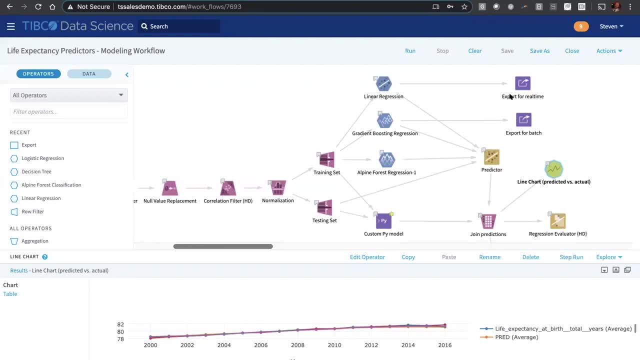 seems to do pretty well, But in any case, we can export some of these models out now for both real time and batch scoring. And what we also did- and you'll see this come into play in a couple of minutes when I go back to the dashboard- we actually filtered down to one country, The 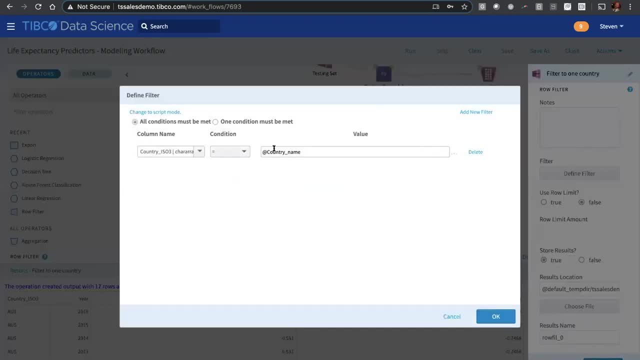 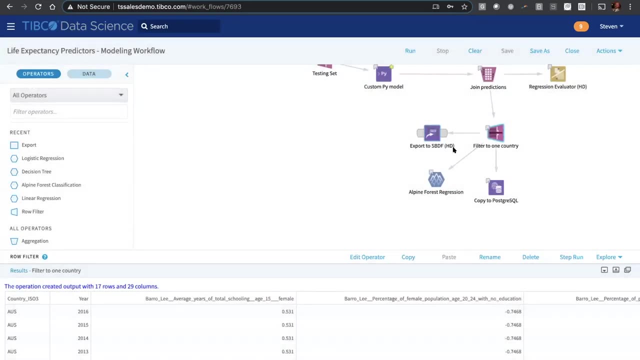 filter here is actually parameterized. So we say the country should equal a past in parameter, which is the name of the country which is going to be, say, Australia or the UK or Ireland, whatever, And then we just build an individual regression there in order to determine what the 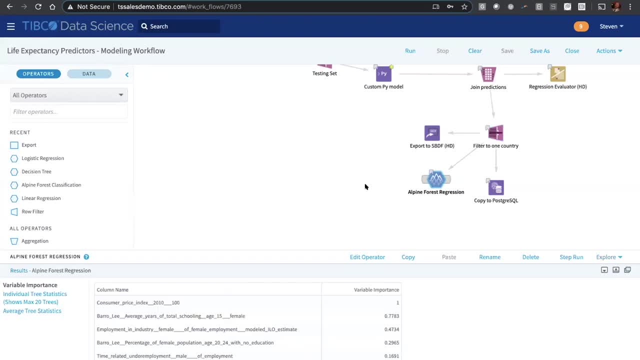 measures of variable importance are for that specific country, And we're going to publish these results back to Spotfire So that we can yield the outcome of this complex workflow, this modeling workflow, back to the simplicity of the dashboard. as you'll see in a second, There are many ways of doing that. 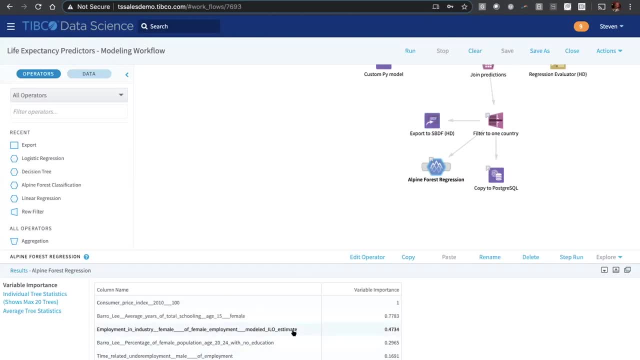 by the way, First of all, you can actually take the output of any one of these operators and surface that directly in the Spotfire dashboard using the data function Michael mentioned. You can also emit a data file that is going to be ready for reading by Spotfire in Spotfire format. 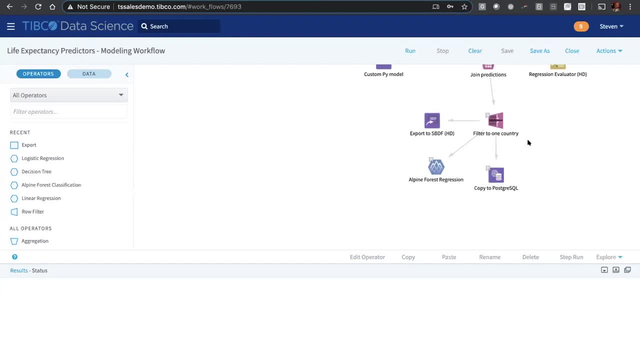 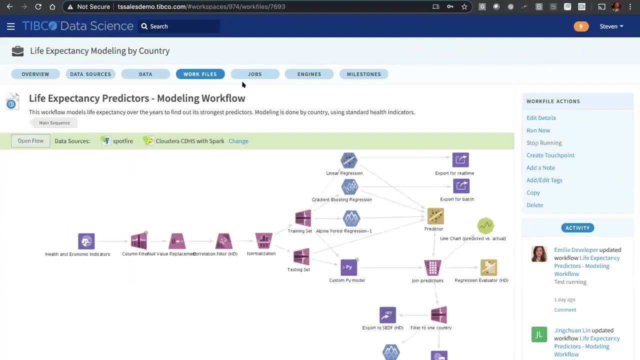 or you can just write it out to a database and Spotfire can access it. So if you read the data out, you can access it through its database interactivity. So I'll get back to that in a second. There are other methods of deploying models that I just want. 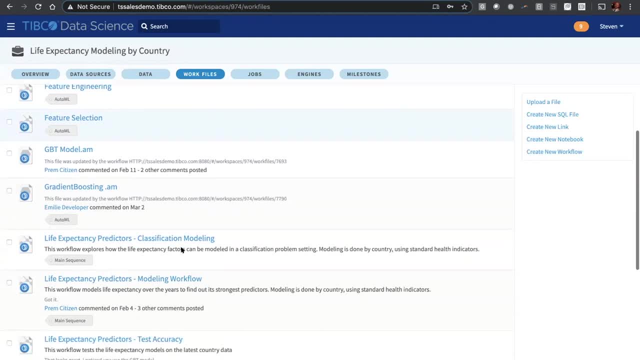 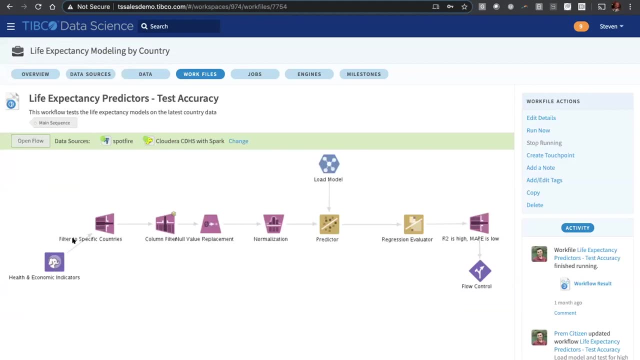 to mention that we could have used. As I said, we're focused really just on deploying back to Spotfire, But here's one method, for example: we can export those models, as you saw me do with that linear regression. We can load that up and use it for batch scoring. So here's a very simple 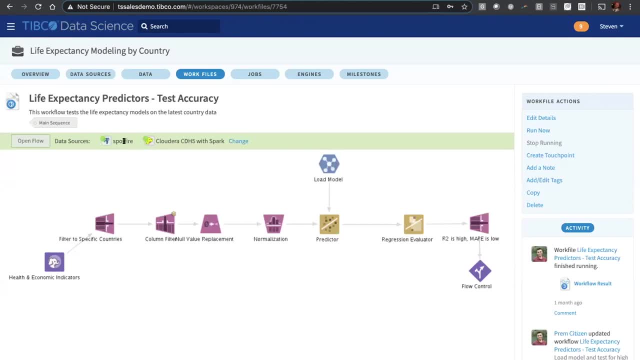 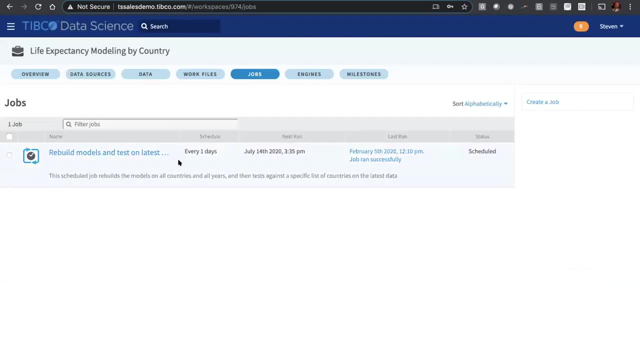 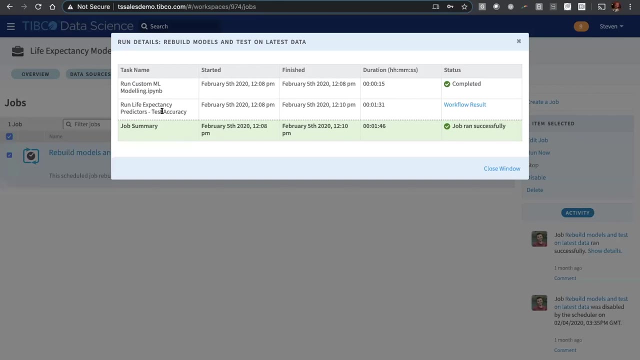 way of doing batch scoring. You can load a model that was developed on Hadoop and deploy it to that for model deployment here for batch scoring. I can then schedule that workflow Here we have a workflow that runs every day. It runs two workflows, some custom modeling in Python. 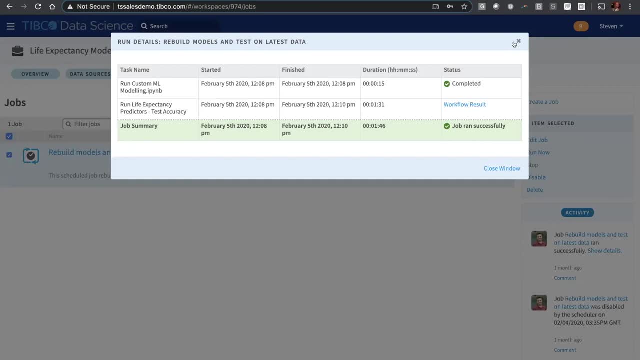 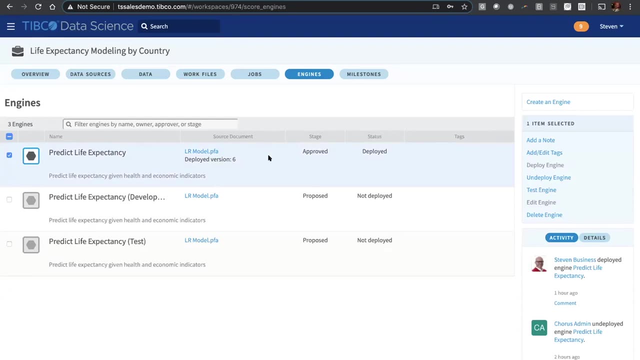 and then the workflow that I just showed you and that can be scheduled. We can also run for real-time scoring. Here is an engine that I have ready, and this is simply taking an export of one of those models that I built- and it literally the click of a button. 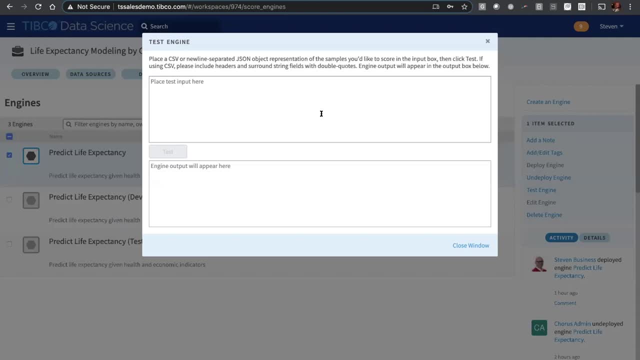 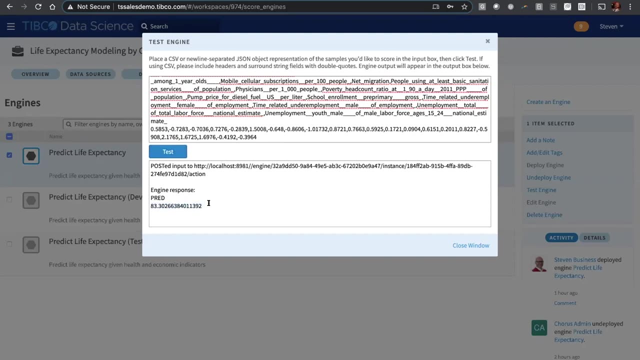 I can deploy that engine as REST service, and now it's available here. I think I've copy-pasted some data here, so this is just passing in data for a particular country and you run it and it gives you a prediction of about 83 years old for this particular country. 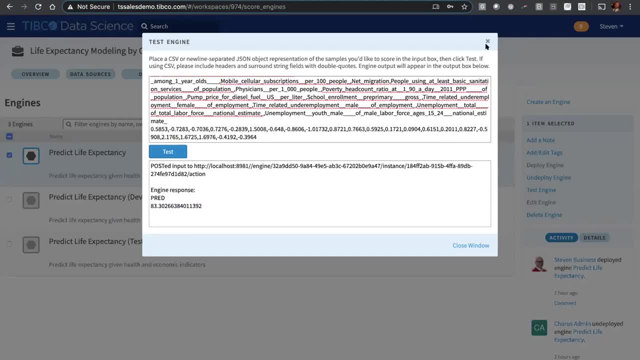 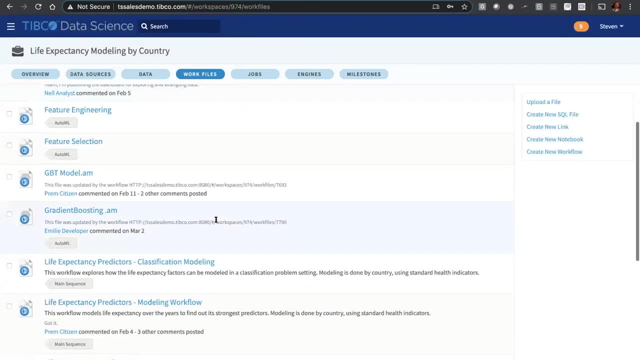 which I think is Australia, So very easy to deploy for both real-time batch scoring. Before I head back to the dashboard and show you how we interact from that, I just wanna mention one other thing. I mentioned that Emily was building these Python notebooks. 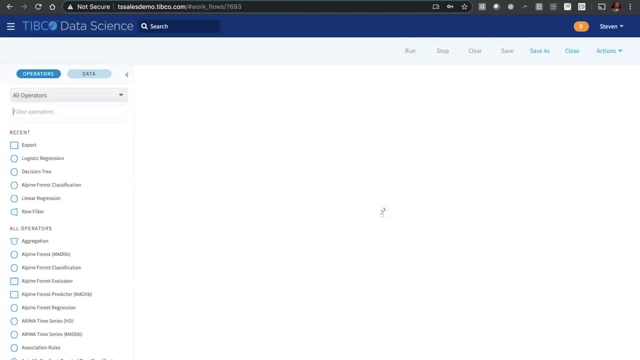 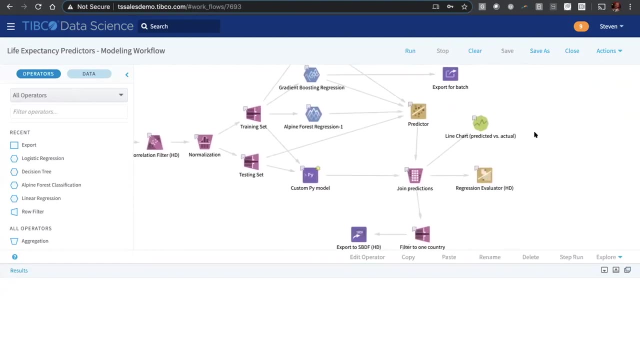 and you'll see. in fact, although I use mostly Python, I use Python to build these out-of-the-box modeling operators for building the regressions. That's what Prem did. He also asked for an Adaboost model, and Emily had a particular version of that. 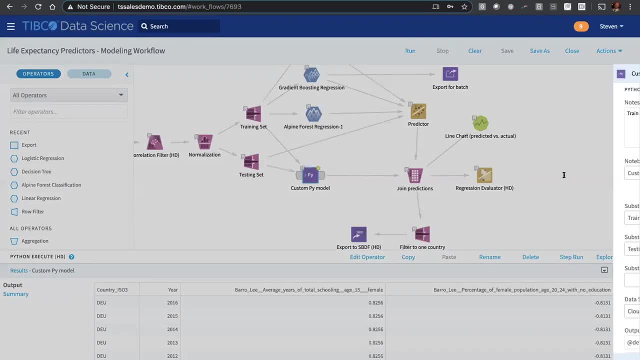 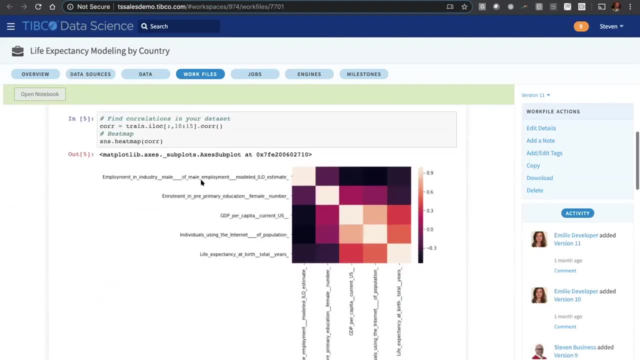 that she had in scikit-learn and so she coded that up in this Python notebook. This is a Python execute model. It's actually run using what it does. it runs this Python notebook here. it is that Emily developed here. 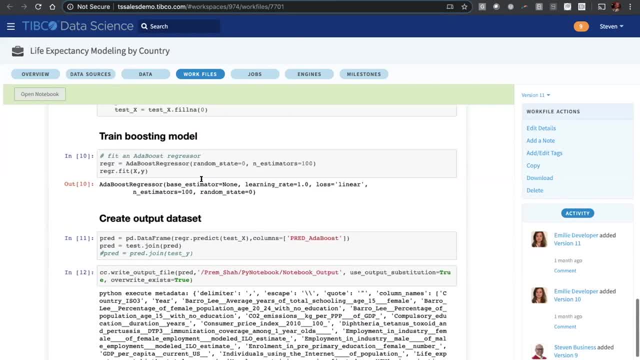 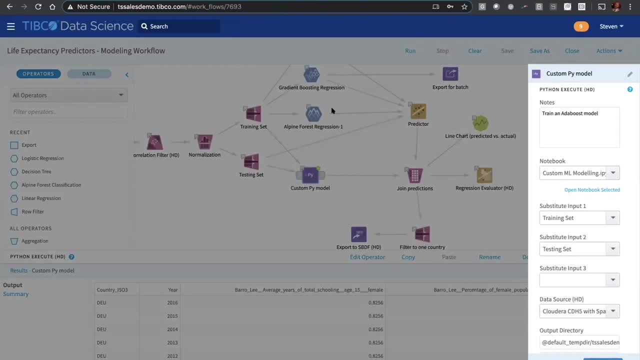 that builds the Adaboost model and ships the results back, So it's a very, very easy-to-use model. It's not as easy as you would any other Python notebook, but because this is operating within TIBCO Data Science, we're able to analyze that code. 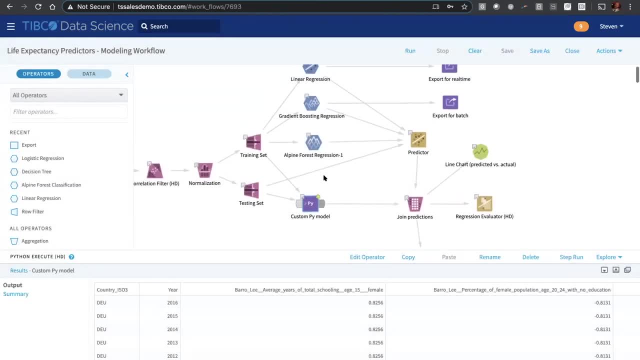 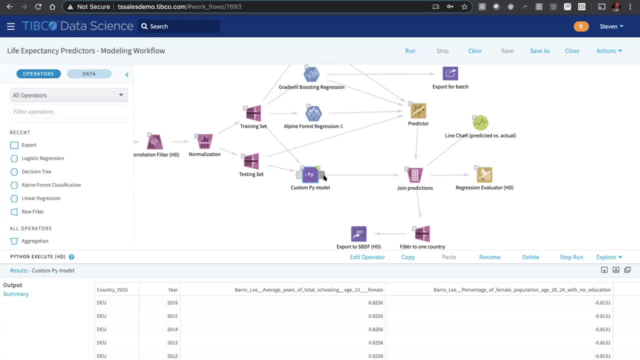 and make it available as a node for Prem to execute within his visual workflow. So a really nice integration there, notebooks being callable from visual workflows and, as it happens, vice versa. Anyway, the point was we developed these measures of variable importance. 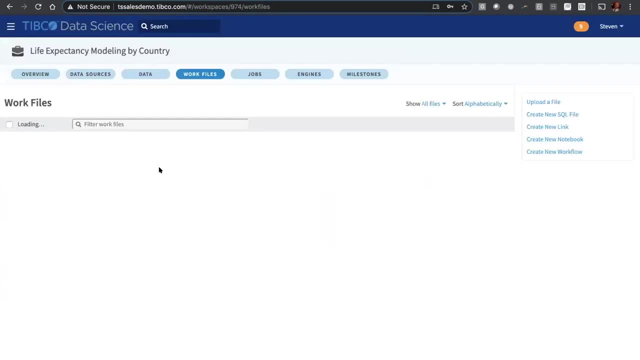 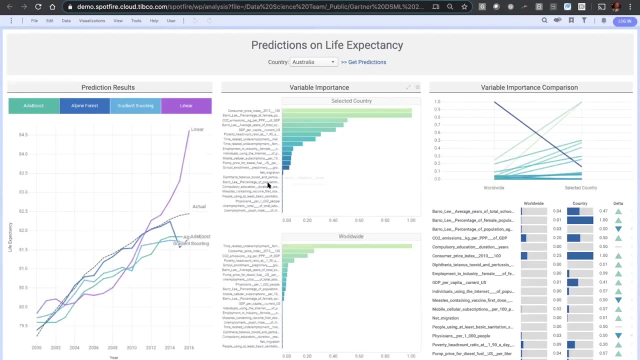 in this workflow, and it was then very easy for us to ship those back to Spotfire via the data function that Michael mentioned. So let me open up this dashboard once more, And here's the result, And this is what Neil did. 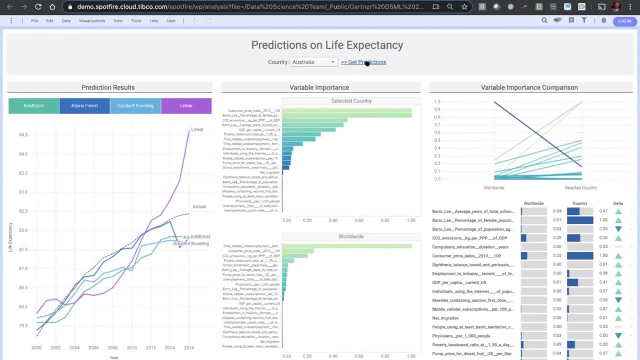 Neil actually managed to build a simple interface here into the TIBCO Data Science platform using our big data function, as we like to call it, And that executes the visual workflow on the backend in TIBCO Data Science and then produces the results. 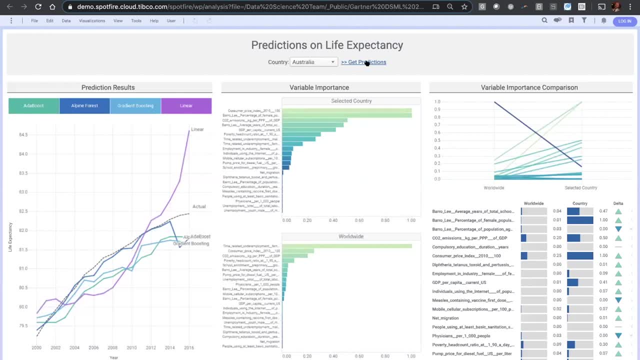 yields the results back to this dashboard, So it's very easy to use. It's very easy, then, for the data scientist to work within the visual workflows and Python notebooks but then to make those results available back to the business analyst- Neil in this case. 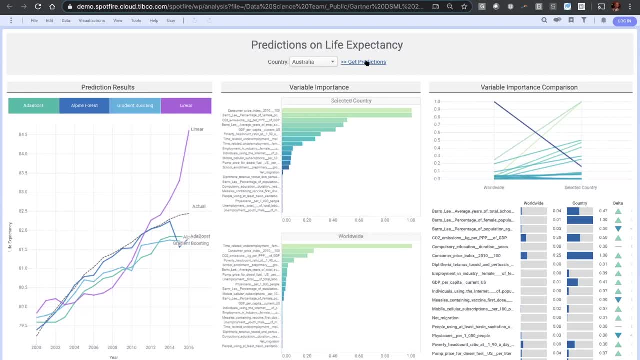 for viewing within the dashboard, Oblivious essentially for a casual viewer of this dashboard that what it's actually doing is running these complex workflows in the background. So here you see, for example, the results of the modeling. You might not typically have this in the dashboard. 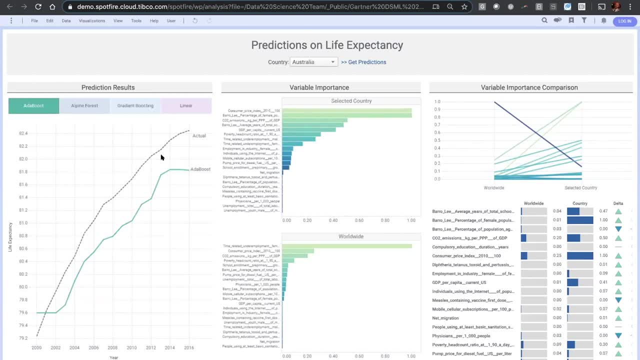 but you can see here the results of the predicted versus actuals that we were building in that workflow. Here the measures of variable importance for a particular country, in this case Australia, versus worldwide. And here's another way of viewing that. On the left, the measures of variable importance. 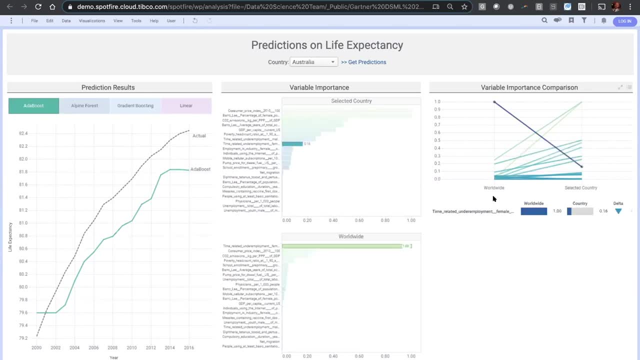 for the worldwide models versus the country-specific model. So you can see, for example, this variable, which is female underemployment, is much less significant for Australia than it is worldwide, Whereas, on the other hand, if you look at these two variables here, 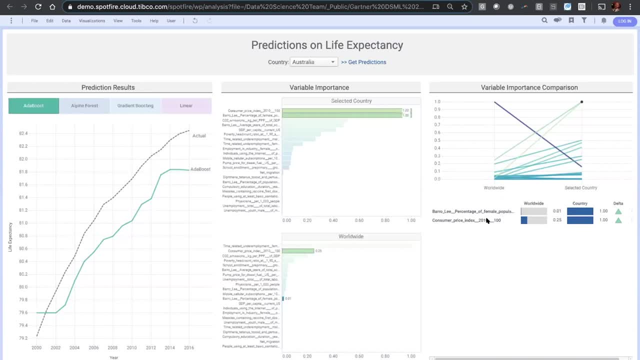 so that's the percentage of the female population that's being used for education, as well as the consumer price index, are particularly important for Australia and perhaps less important in general for other countries. So very easy for me to use the power of Spotfire. 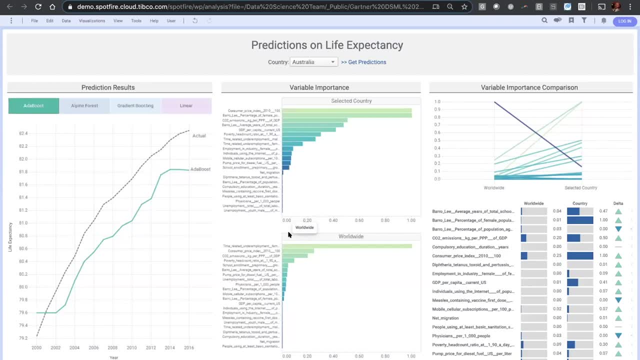 here to explore my data, both on the front end, to get used to it, to figure out what questions I want to ask, to then pass that on to the data science team for producing more sophisticated analyses, and then back to the dashboard to yield the results of those analysis. 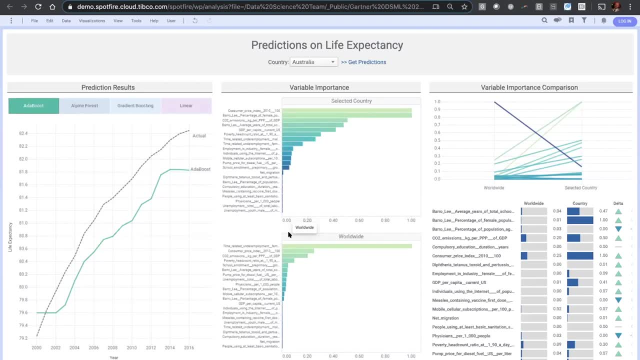 for the business analyst. So I hope that makes it at least a little bit clear how those different personas can interact with each other through TIBCO, Data Science and Spotfire and to build an integrated analytics pipeline from data prep all the way through to predictive models. 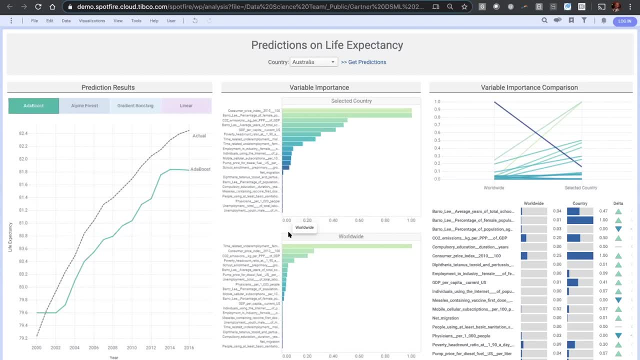 that can be deployed in batch or real time and then ultimately out to visual applications.